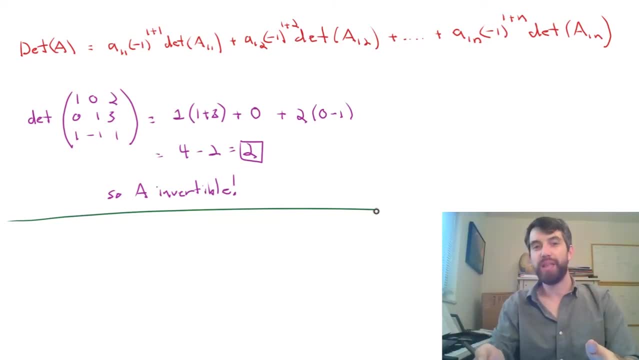 We've seen that we can apply this determinant formula where it is so-called expanded along the first row, because my aij's always were a1j and that was my expansion along the first row. This general process that we're doing, it actually works, expanding along any row. I didn't have to. 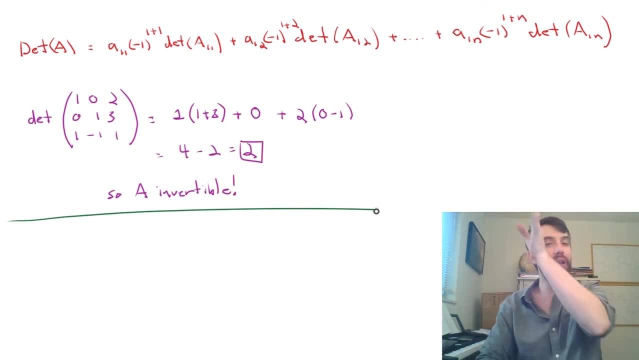 put a 1 in there And it also works expanding along any column. So I'm going to do precisely what we've done before, but this time I'm going to do the determinant: not expanding along the first row, but expanding along the second column. If we wanted to, we could write out our whole big 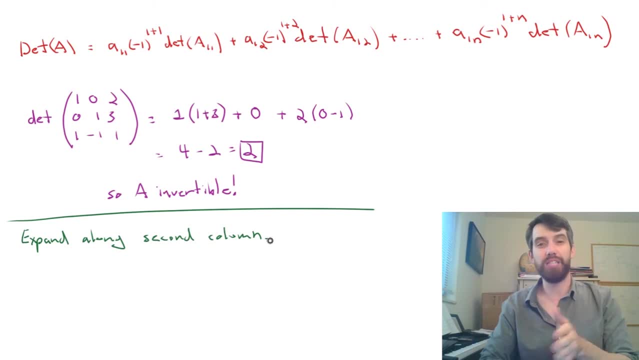 formula where we're leaving the first components, the i's, unspecified, but the second component, the j's, are always fixed at being equal to 2.. But I don't think we need to do that, By the way, since you can expand along any row or any column. 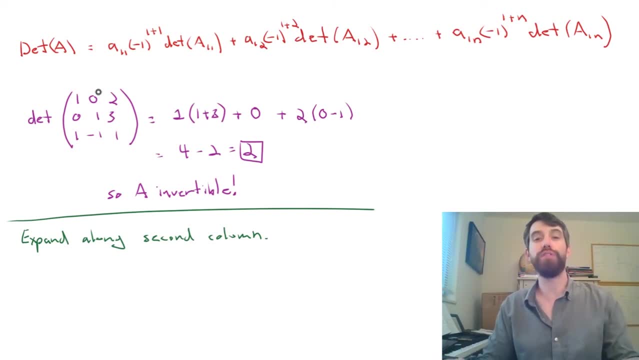 it's basically no problem if you expand along any column- usually helpful to expand along a row or column that has a lot of zeros. It turns out for this particular matrix you've got a couple rows or columns that have some zeros in them and 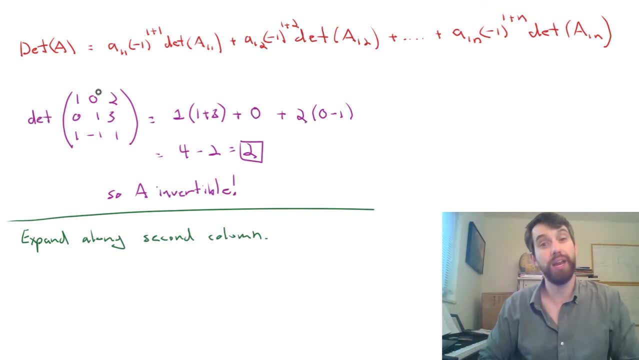 expanding along. the second column is one of the ones that has a zero, so it's kind of nice, Okay, so what am I going to do? I am going to be going down this main column, so that's what I'm going to be going. 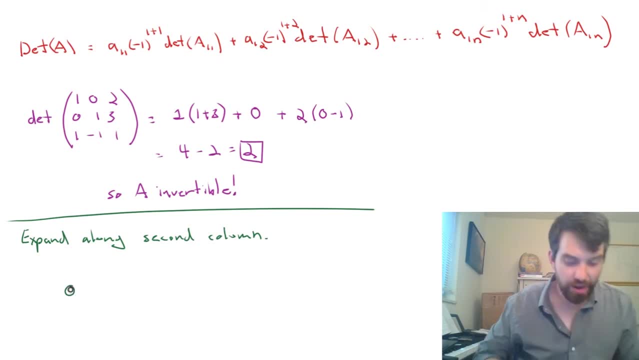 down And my first part is right there in the A location, I have a big fat zero, so I start that off. I don't even worry about my minus ones, I don't even worry about my determinants, because they're all going to multiply by zero. Next up, I'm going to be looking here. 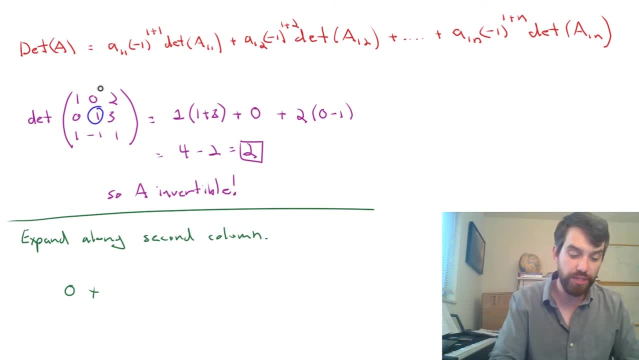 at this one right there. That's my next step if I'm going down this particular column. Alright, so that's going to give me a value of one. It's going to have a minus one to the two plus two, which is four, so it's again not going to have. 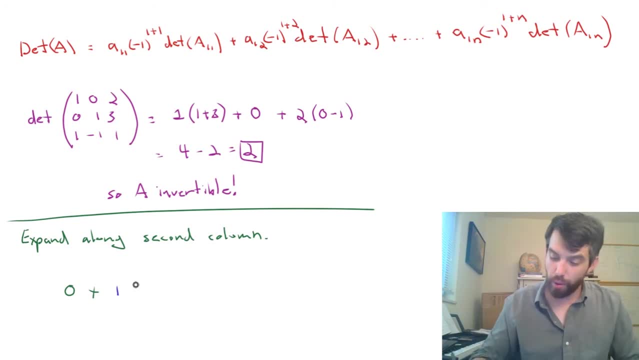 a minus one, so it's just going to be times one. I won't put anything in. And now I want to worry about the determinant. but we have to be a little bit careful here, because A22 is the matrix that gets rid of those two rows and columns, And so that leaves me.